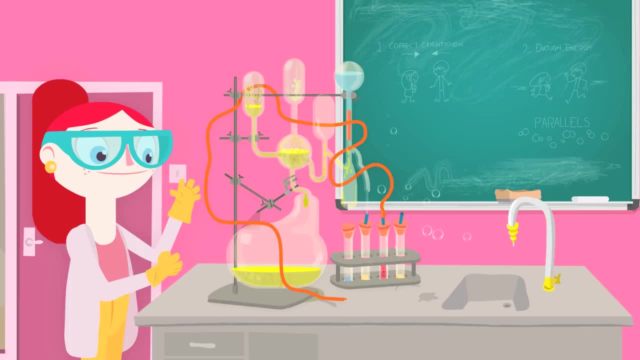 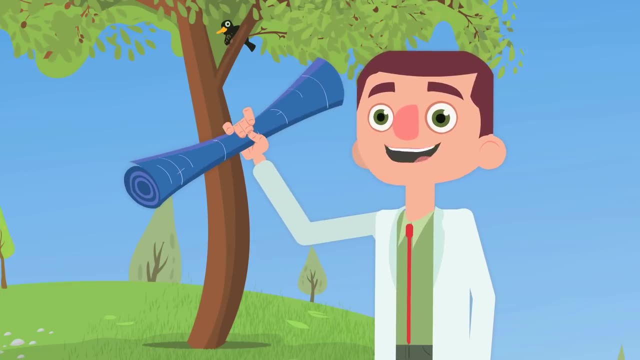 we decided to set out on two missions. Harriet wanted to help all chemistry students and chemists remember how to speed up the rate of chemical reactions and I, being the nice guy that I am, decided to make it my mission to help create educational environments in. 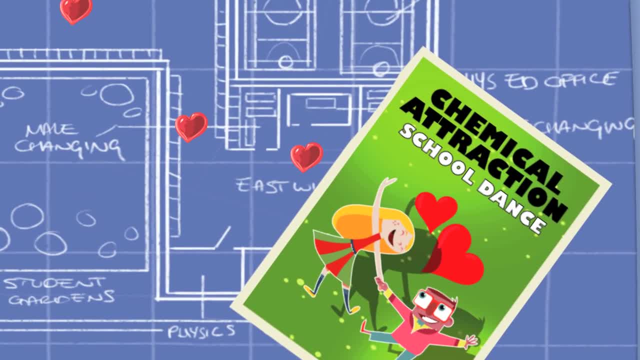 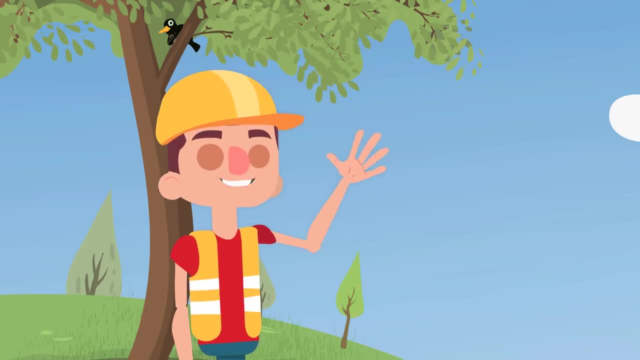 which more book-dropping collisions can take place. to increase future chemists' chances of getting a date for the dance, In order to facilitate this improved dance date-getting process, I propose five changes to all schools that parallel Harriet's five ways to increase chemical reaction rates. 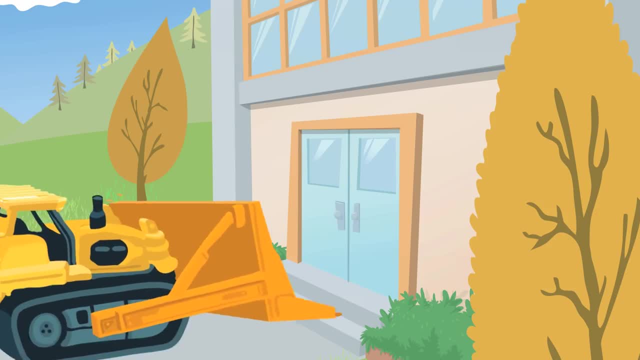 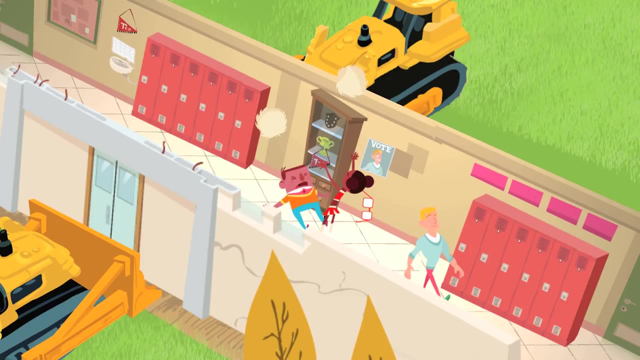 First, I propose that we shrink the size of the hallways. This will make it more difficult to safely navigate the hallways and will cause more collisions than in larger hallways. And by increasing the number of collisions we increase the likelihood that some of those 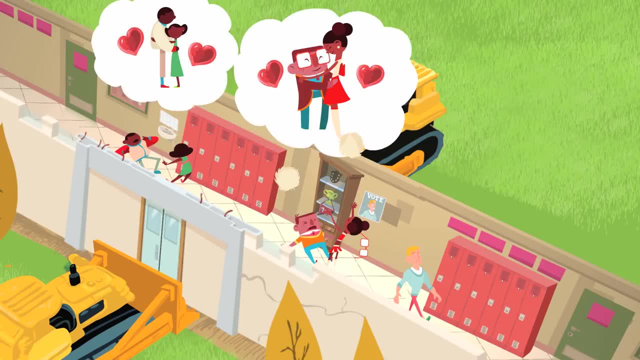 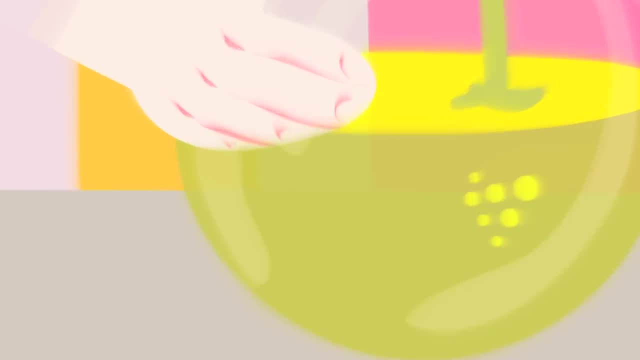 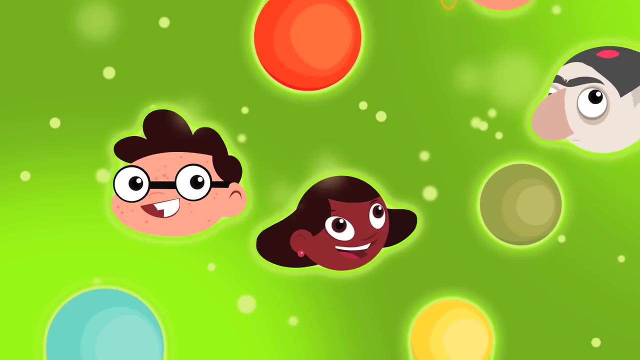 collisions will have the correct alignment and enough energy to create a date to the dance. Basically speaking, this is equivalent to lowering the volume of a reaction vessel or a reaction mixture. In doing so, the individual particles are closer together and more collisions will occur. More collisions means a greater likelihood that collisions with the appropriate 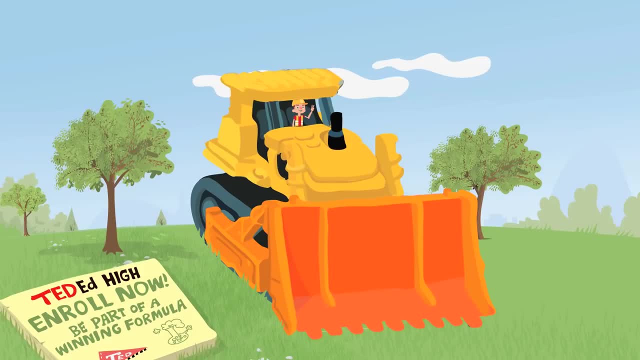 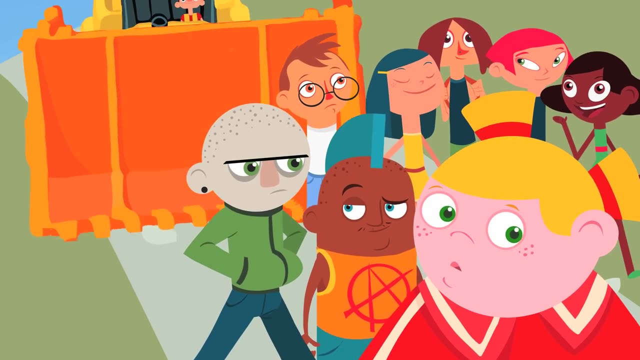 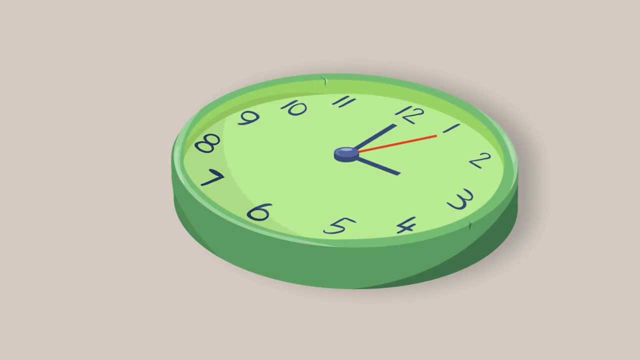 energy and configuration will happen. Second, I propose increasing the overall population of the school. More students equals more collisions. By increasing the number of particles available for collision, we create an environment where more collisions can take place. Third, we reduce the time allowed between classes. Heck, let's just cut it in half. In doing 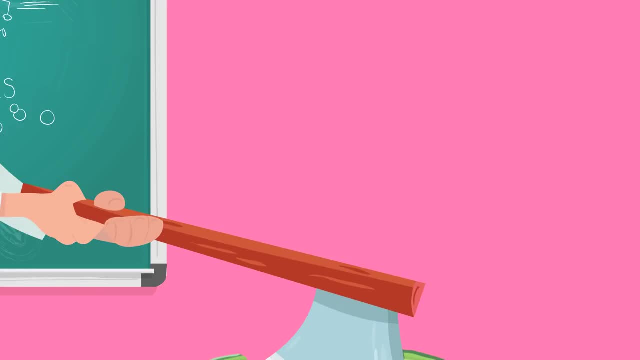 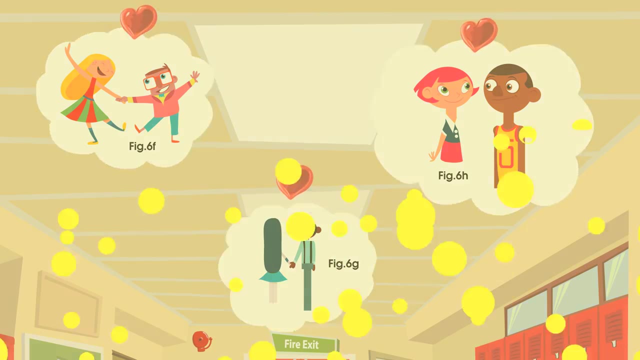 so students will need to move more quickly to get from one class to the next. This increase in velocity will help make sure collisions have the appropriate amount of energy necessary to ensure book dropping. This is analogous to increasing the temperature of the reaction mixture. Higher temperature. 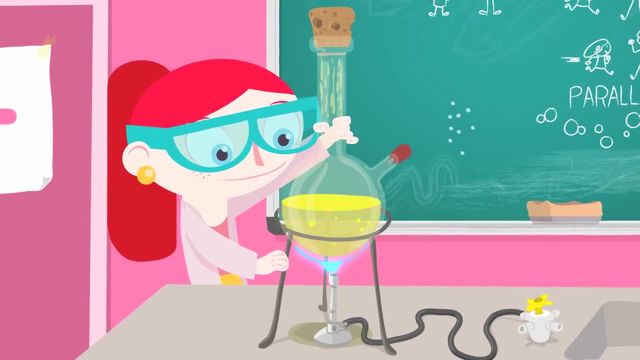 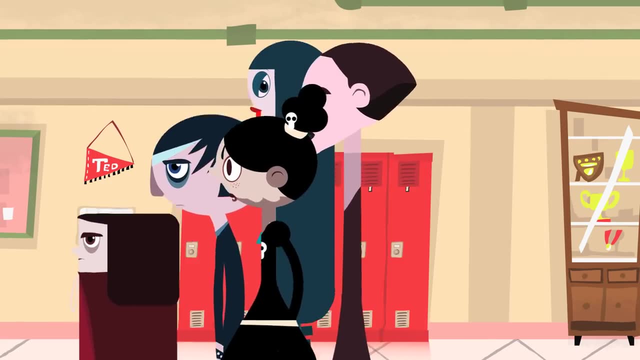 means particles are moving faster. Faster moving particles means more energy and a greater likelihood of reaction causing collision. Fourth, students must stop traveling in packs. By traveling in packs, students will be able to move faster. This means that they will be able to move faster. This means that they 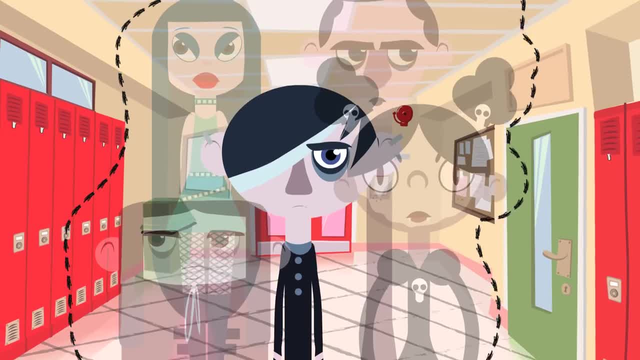 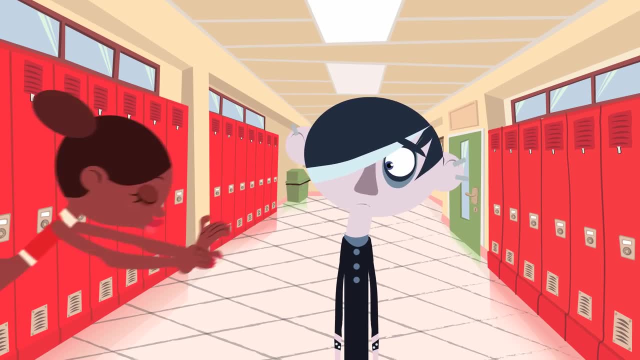 will be able to move faster By traveling in packs. those students on the outside of the pack insulate those in the middle from undergoing any collisions. By splitting up, each student has more area exposed that is available for a collision from a passing student. 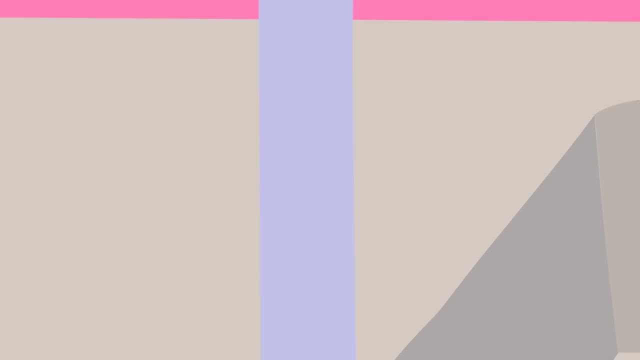 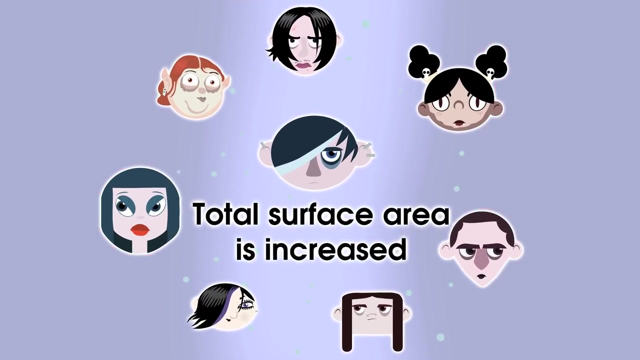 When particles travel in packs, the surface area is very small and only the outside particles can collide. However, by breaking up the clumps into individual particles, the total surface area is increased and each particle has an exposed surface that can react. Fifth,